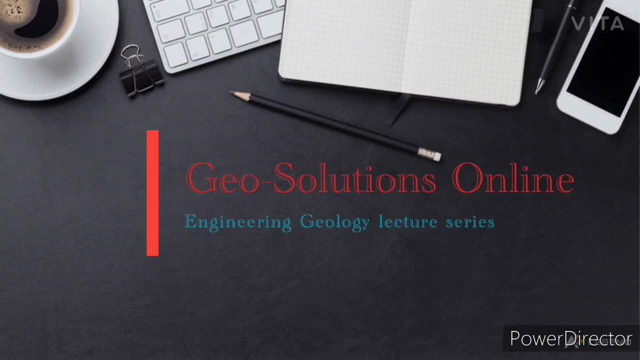 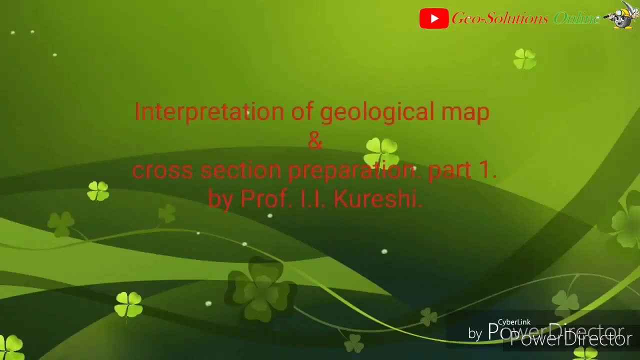 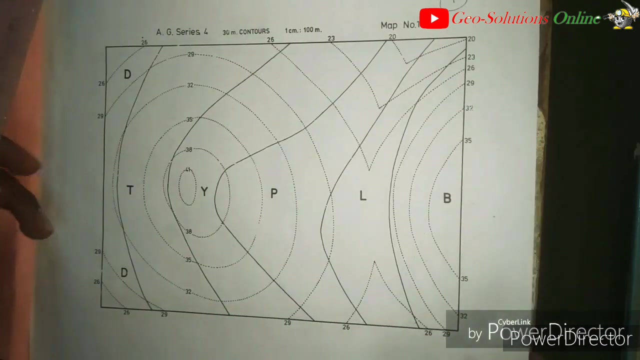 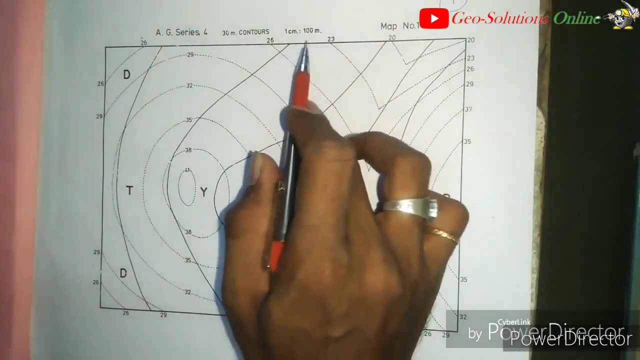 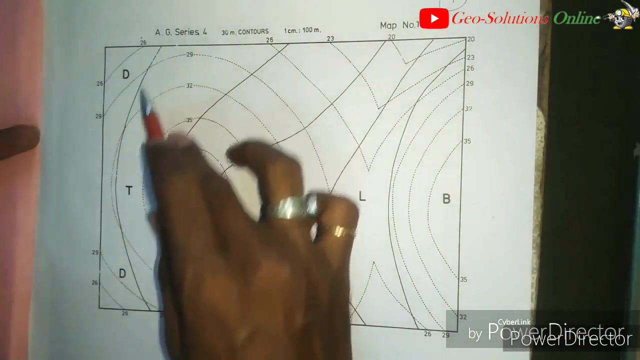 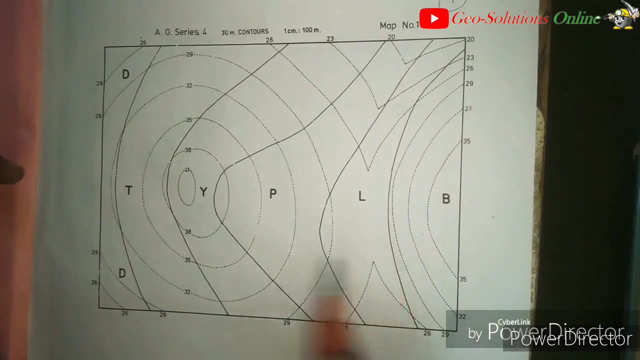 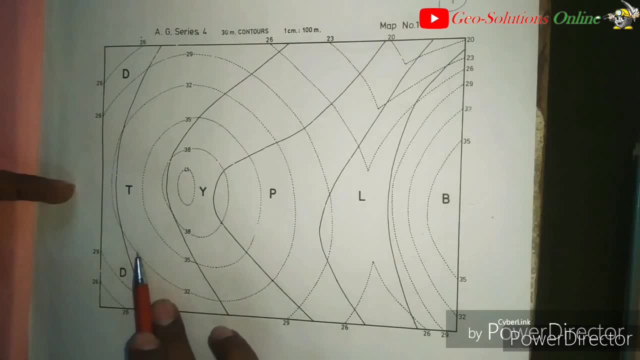 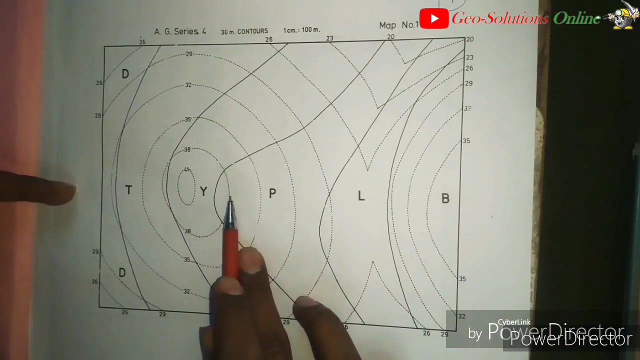 which is having boundary of D as well as T beds. okay, and this is Junction DY, because this is having boundary of D and boundary of Y. this is Junction YP, because same this is having boundary of bed Y and bed P, and so on. PL, LB- okay, this. 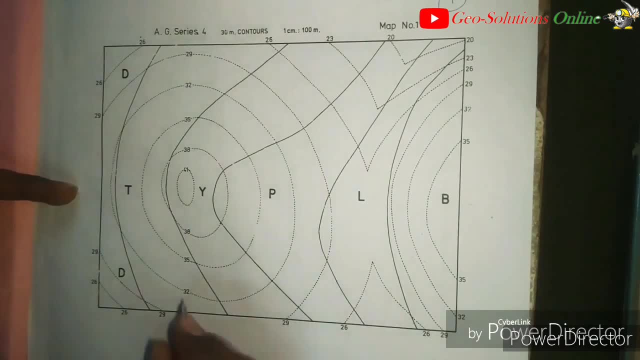 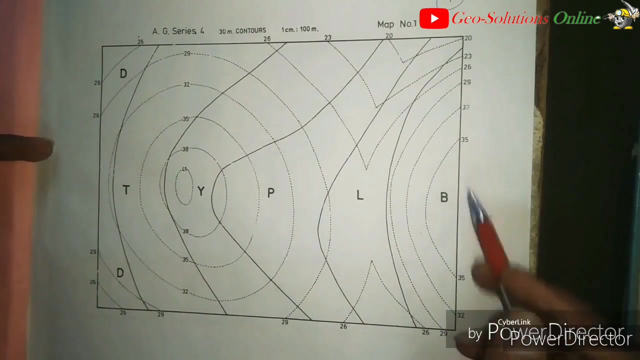 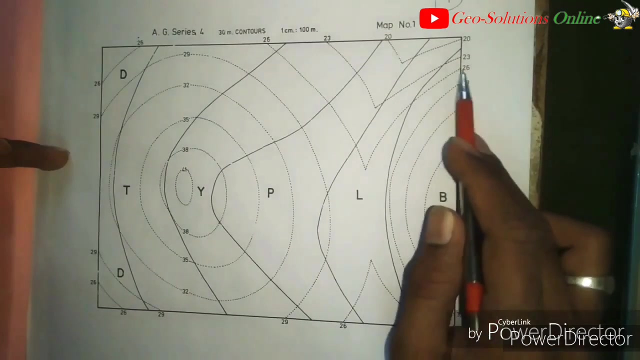 dotted line is having some values, that is this values, which is contour lines. okay, this contour lines are in semicircular form here because it is showing contour of 350 meter, 320 meter, 290 meter, as well as 260, 230 and 200 meters. this contour lines are: 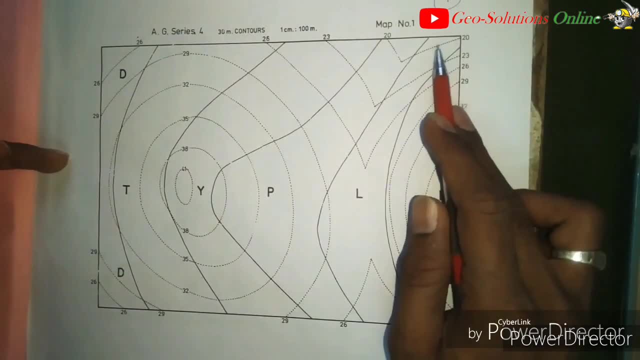 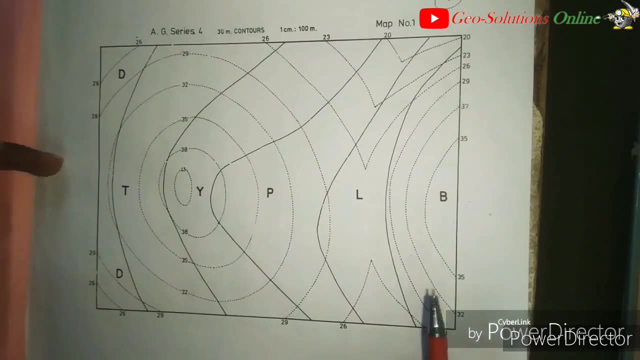 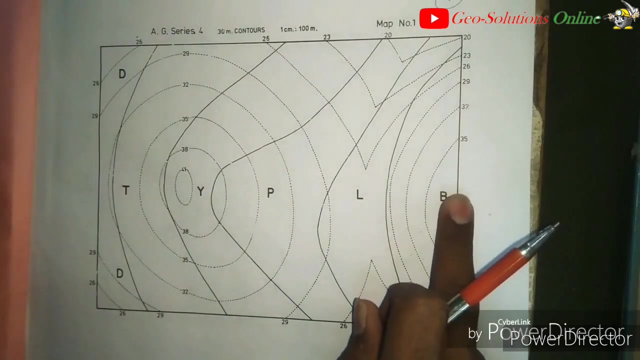 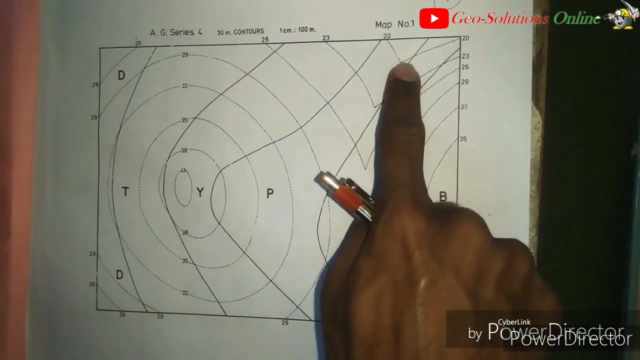 making V shape because it is having a valley here in this side of the map and second valley in this side of the map because this, geographically, this map contains a one isolated hill and a portion of another isolated hill, and this isolated hills is giving rise to valley number one and valley number two and 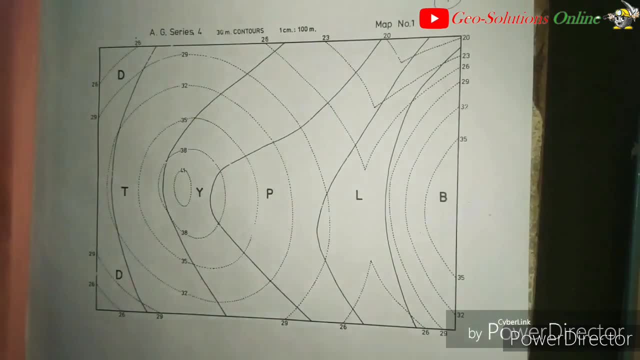 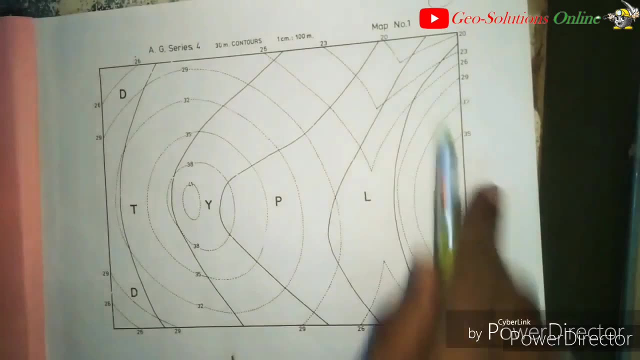 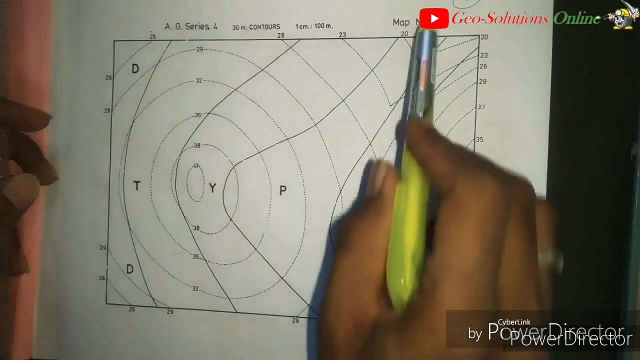 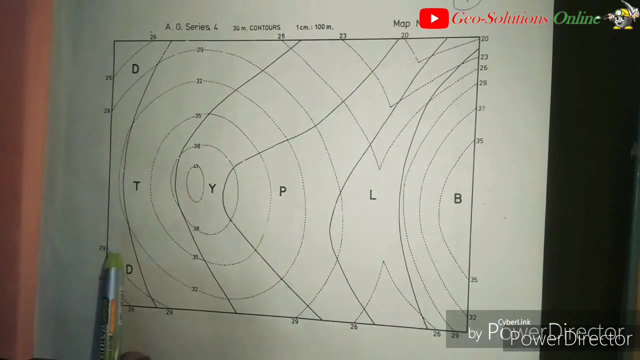 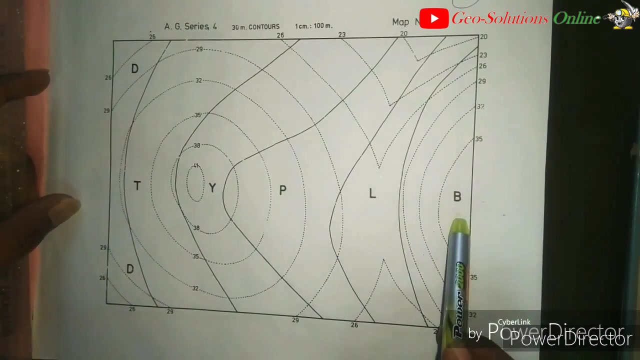 these. if a map contains two valleys running opposite direction in this portion is known as a saddle. so geographically, this map contains a isolated hill, a half portion of isolated hill, valley number one, valley number two and a saddle. okay, and this map contains a conformable series of beds: bed D, bed D, bed Y, bed P, bed L and bed P. okay, and it is. 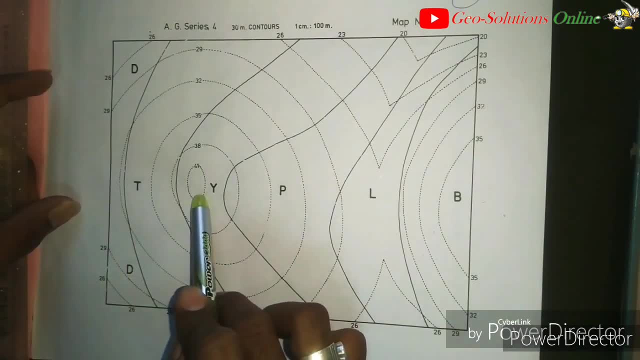 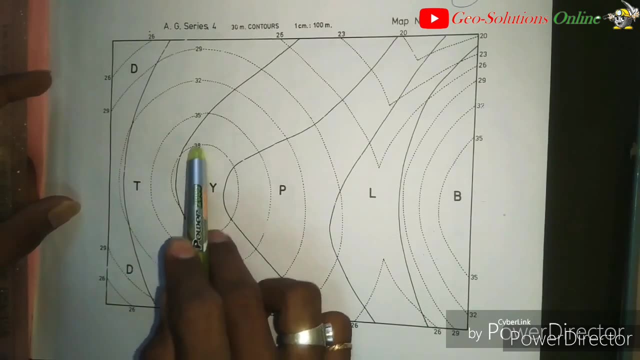 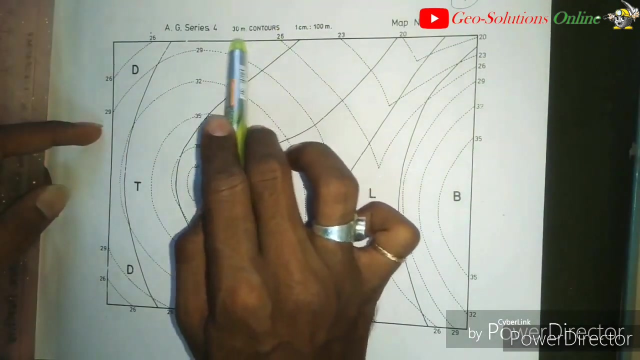 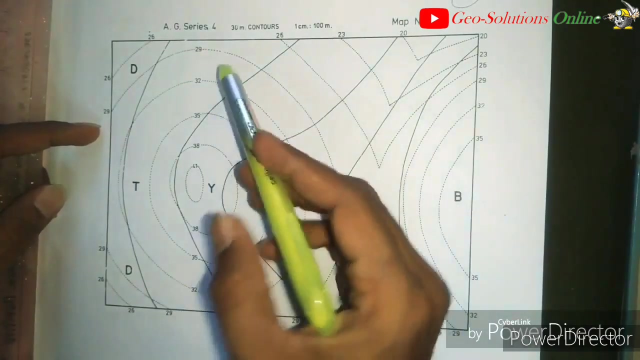 having contours of highest contour, or we can say maximum elevation point of 410 meter and minimum control of 200 meter. okay, given data is: contour interval is 30 meter. scale of the map is one centimeter equals to 100 meter. okay, contour interval means the distance or difference between 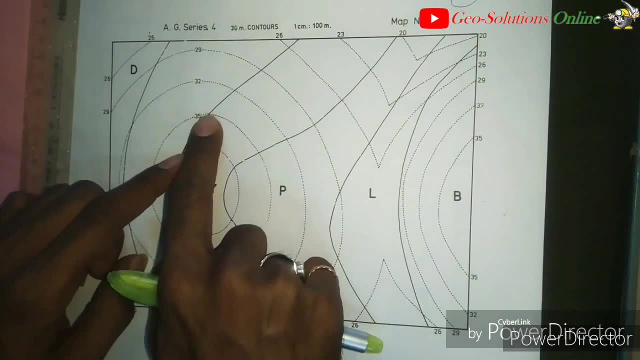 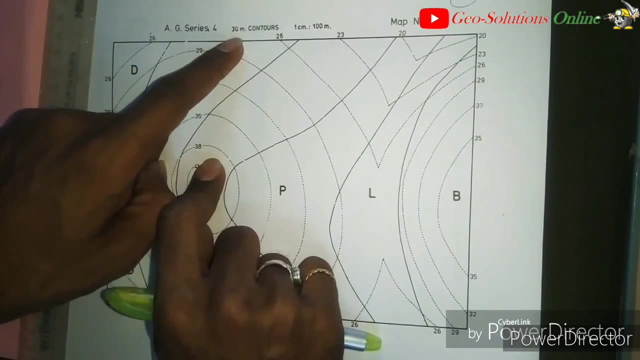 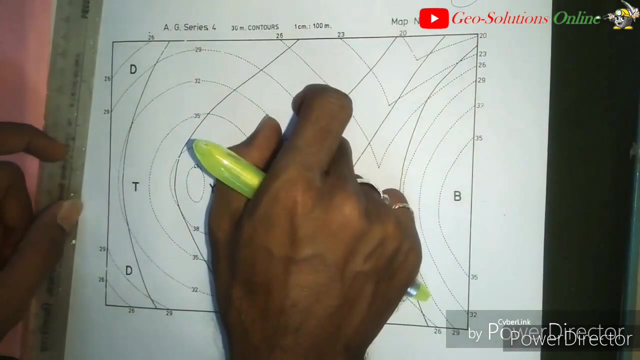 two control. here we can say 380 minus 350, that is 30 meter. difference between two contour is of 30 meter. that is contour interval okay. and the scale of the map is: one centimeter equals 200 meter. that means if we study one centimeter on this map then it will cover actual field. on: 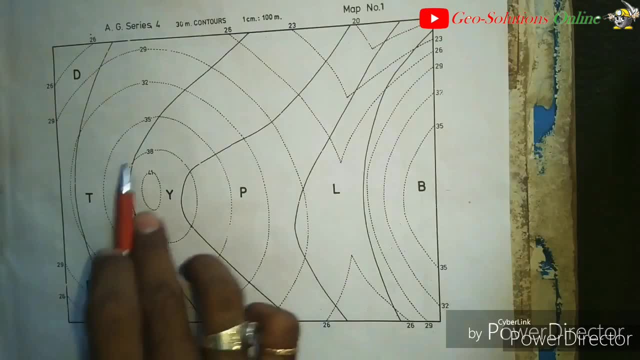 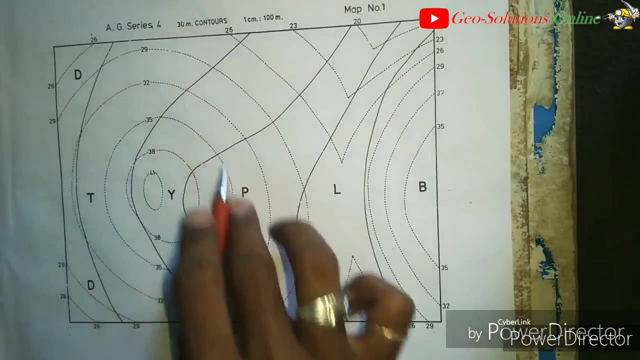 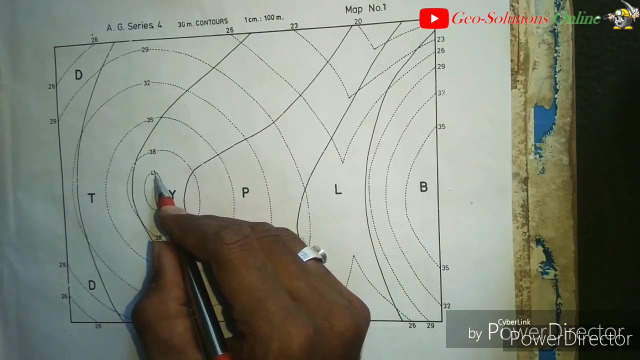 100 meter area. okay, how to know whether this portion is a hill or a depression or a basin, like structure? these contour lines are in a circular shape, semi-circular shape, okay, and this contour lines are having values of uh four: uh 410 meter, 380 meter, 350 meter, 320 meter. 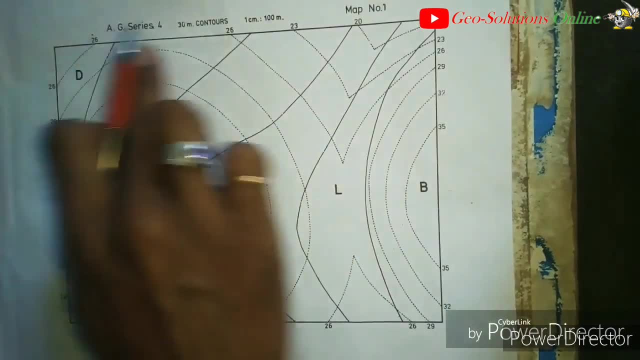 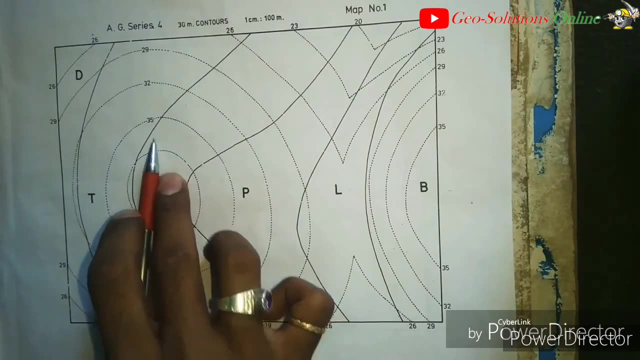 and 290 meter. okay, if this concentric values or this concentric circle is having the value, maximum value, at the center and the value is decreasing away from this circle, that means it is an highly elevated portion or a hill like portion, or dome like portion. okay. and if this value in the center of these concentric 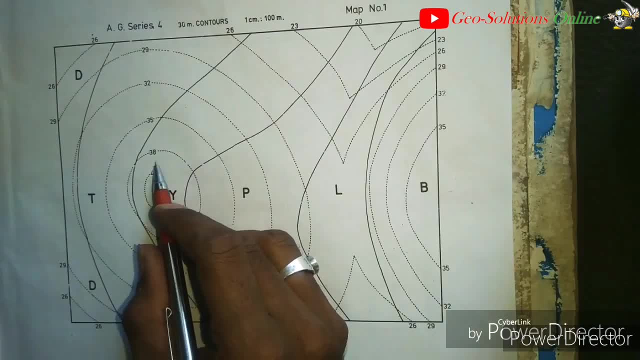 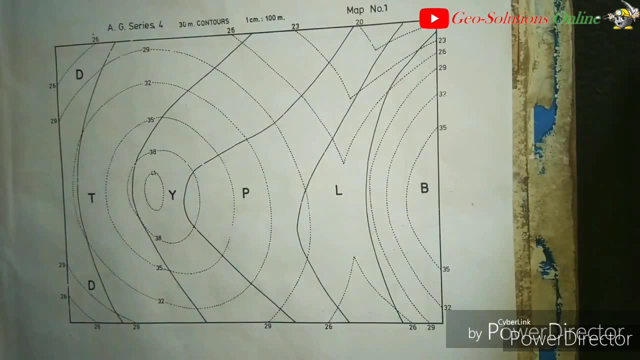 rings. if the center value is less and increasing away from the center of the circle, then that area is a depression like, or basinal structure. okay, so this is a hilly, isolated hill, okay, hilly portion, okay. so first you have to, uh, draw the strike lines on this map for the further. 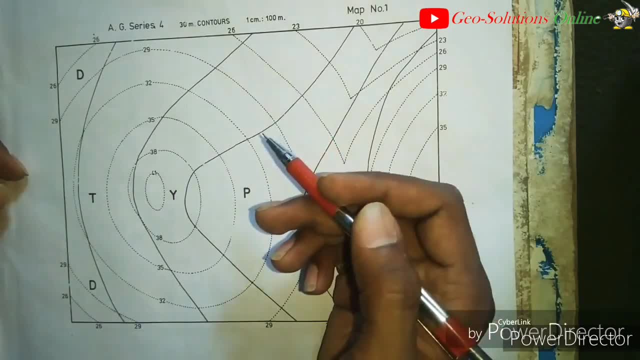 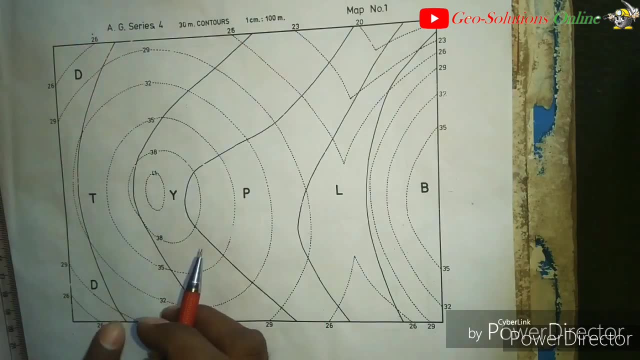 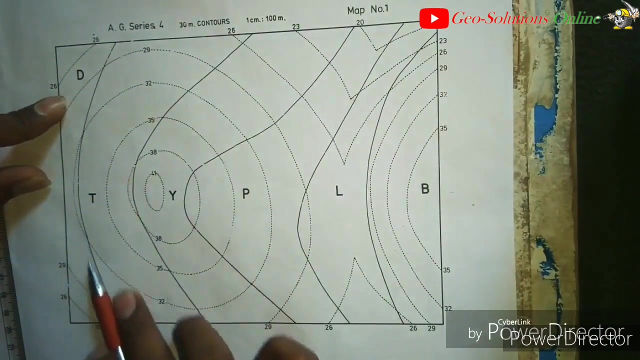 procedure. so how to draw the strike lines. strike lines you must draw. you can see this. this junction is going from this to this boundary of the map and some contour lines are intersecting with this junction points. okay, so where, whenever you have a hilly portion, you have to draw a hilly portion. 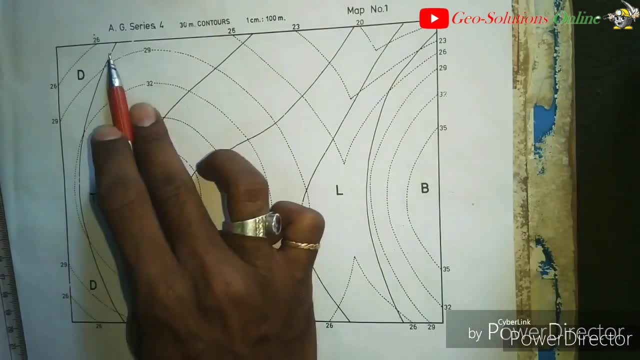 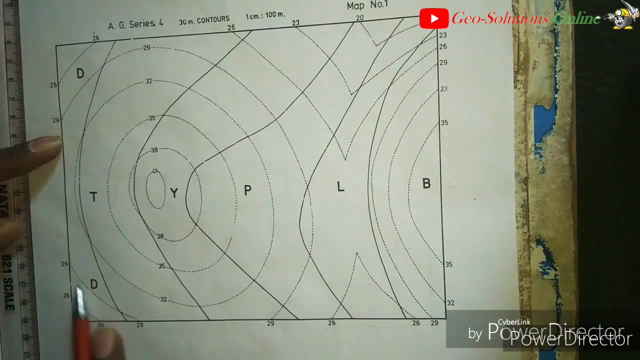 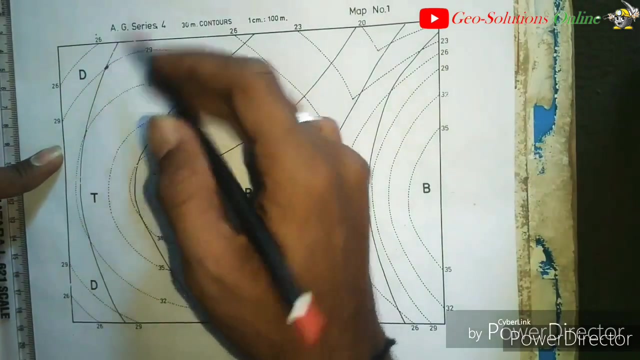 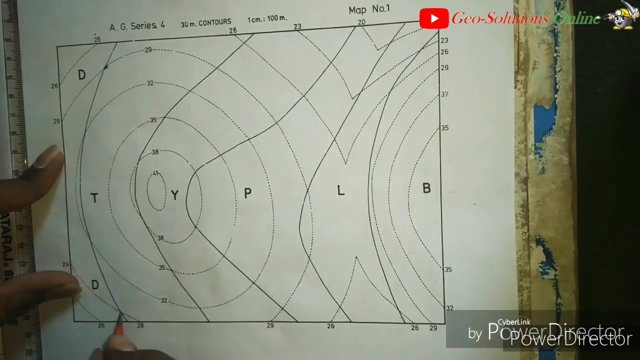 whenever these contour lines are intersecting with this junction point on the same junction line, a same contour line is intersecting, then you have to, you have to mark this point. so this is the junction dt and this is the contour of 290 meter. here also, this is the contour of 290 meter and this is the junction dt. same junction. 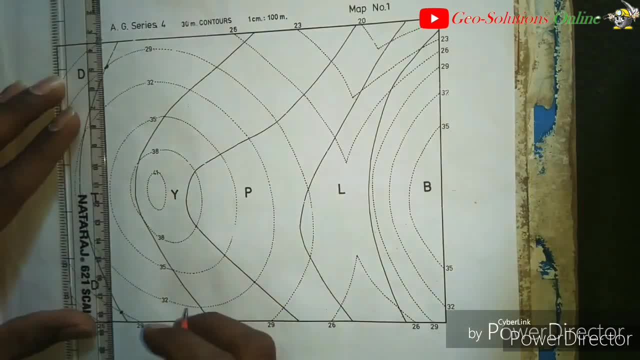 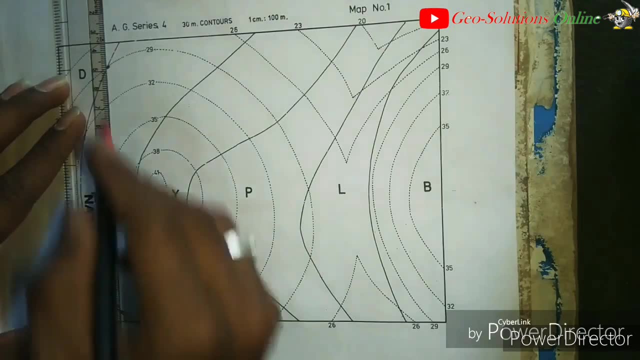 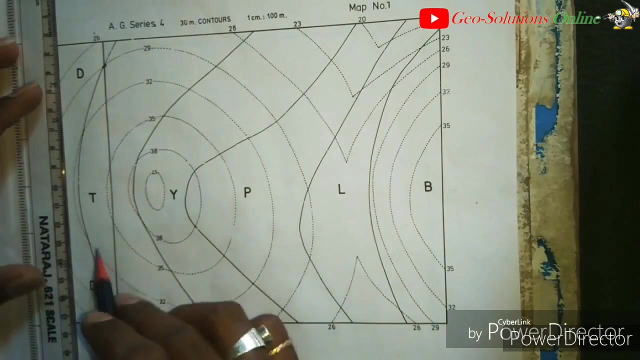 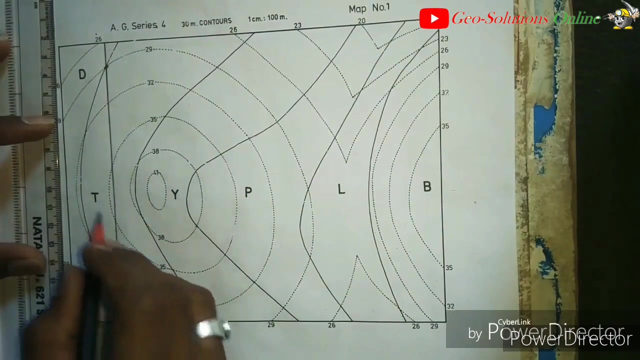 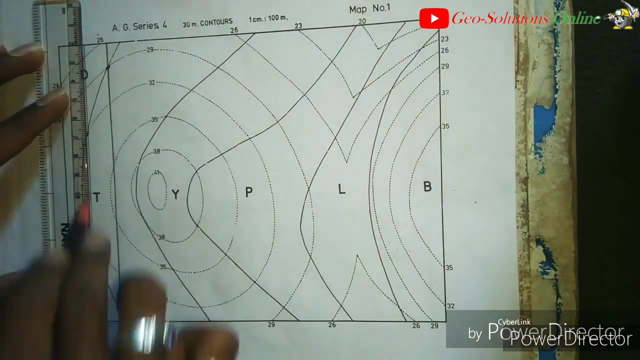 same contour line is intersecting twice, then you have to draw a line on that point of intersection carefully, on same junction contour line of 320 meter. here it is intersecting okay, and same contour line is intersecting here also. so you have to draw a line on that point and join the line. 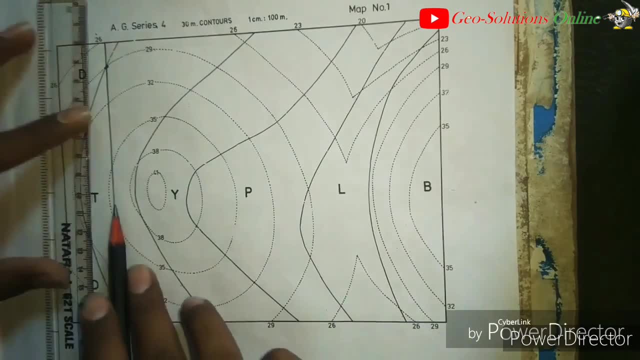 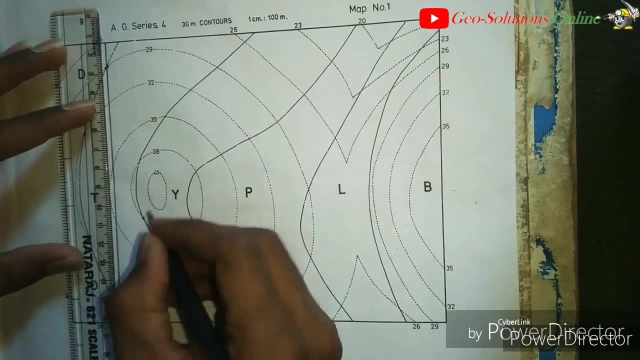 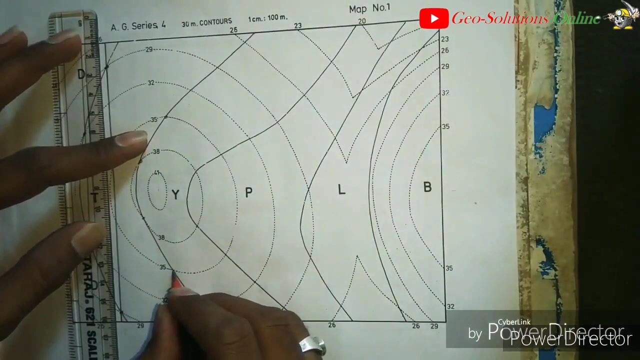 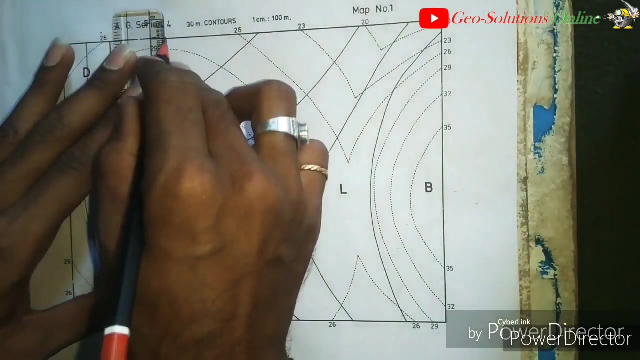 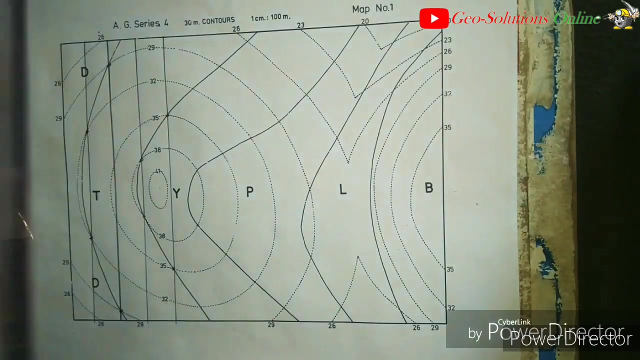 then on this next junction, or bedding plane junction ty, you can see this contour of 380 meter is intersecting here and intersecting here. contour of 350 is intersecting here and intersecting here also. so mark that point and join the line. ok, if you will measure the distance between two successive strike lines, you will get the distance. 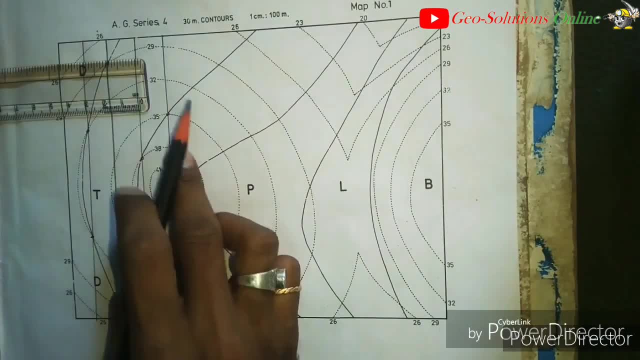 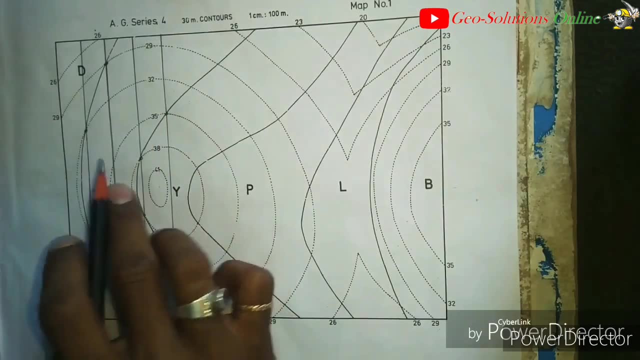 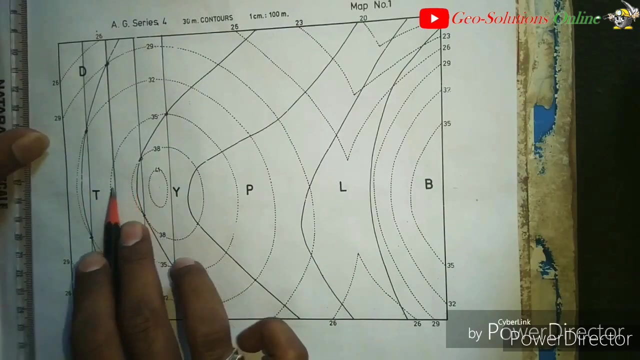 of 1.5. okay, another one, 1.5, same. another one: you can see: 1.5, same. so if you have drawn a two strike lines and the distance between a strike lines is greater than 2.5, okay, you can see that one is larger. 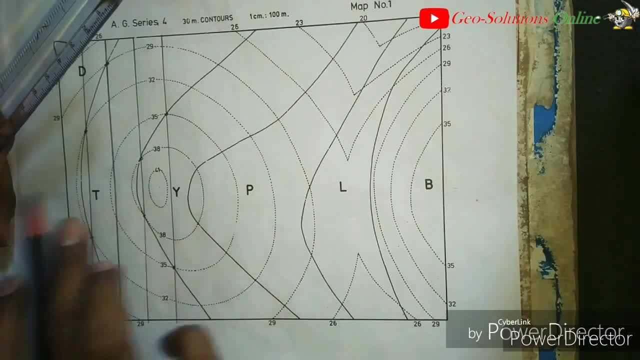 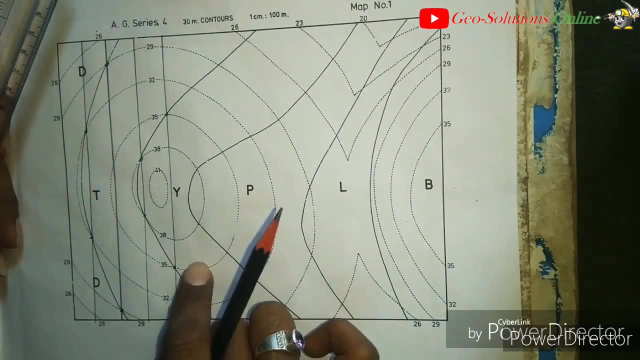 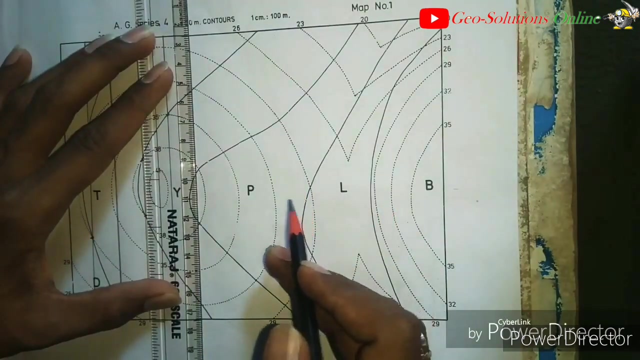 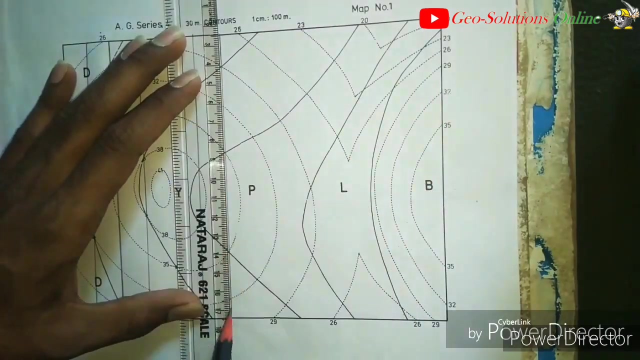 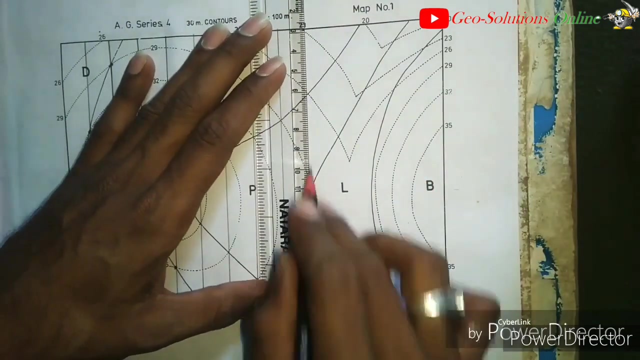 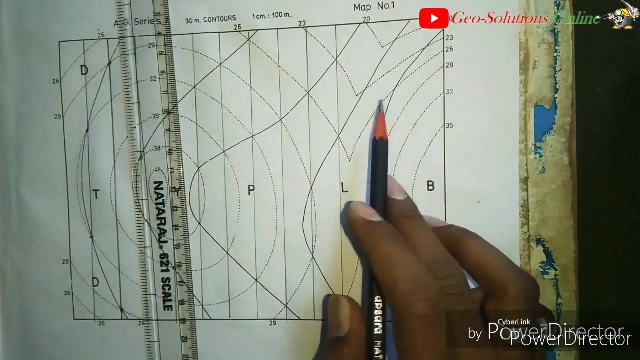 strike line is 1.5 or 3 centimeter, then whole strike lines on this map will be having the strike interval of 1.5 only. okay, so we will join all these intersection point of intersections carefully. sometimes you will finish the case like this: here is a inter point of intersection and the 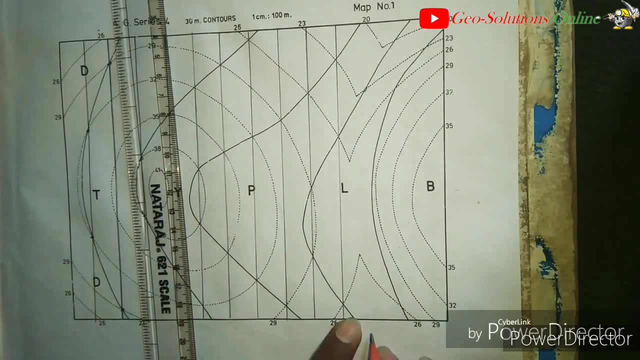 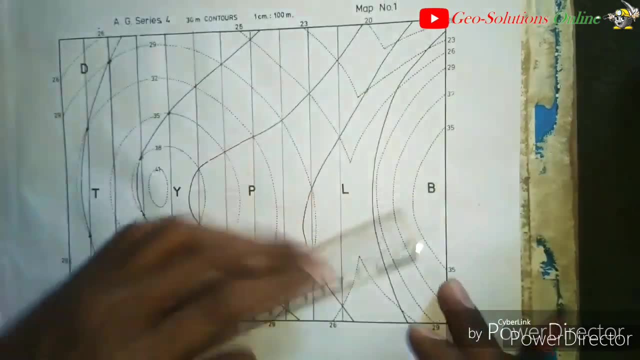 this junction is ended here and we can't get the second point here and the intersection is ended and we can't get the second point and the intersection is ended here and we can't get the second point of intersection, then in that case you have to assume that measure the distance of 1.5. 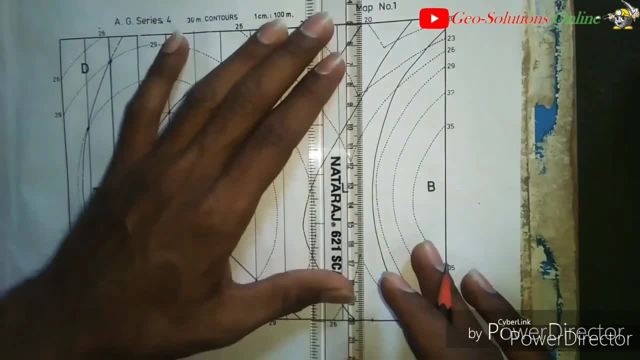 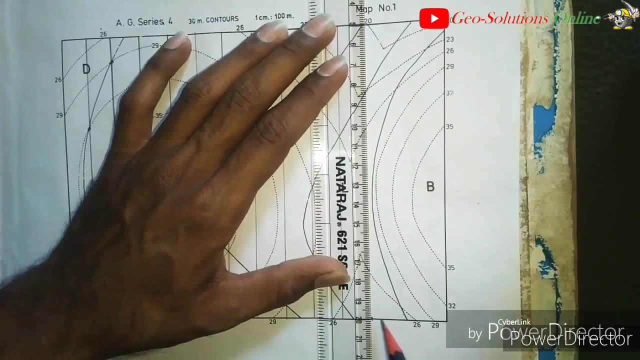 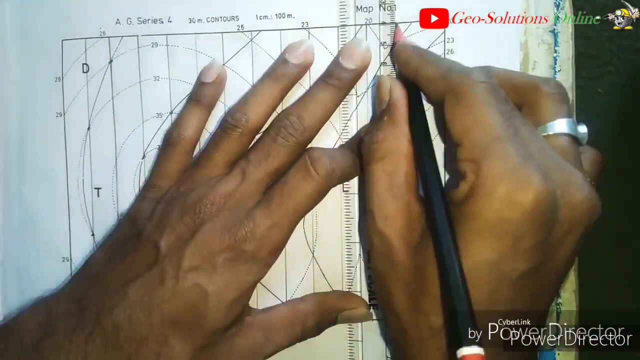 from this strike line. mark it here and join that point of intersection with this marked point of 1.5 centimeter, okay, or whatever the distance between two strike line is. then you will get the strike line okay. so we have already drawn all the strike lines on this map. 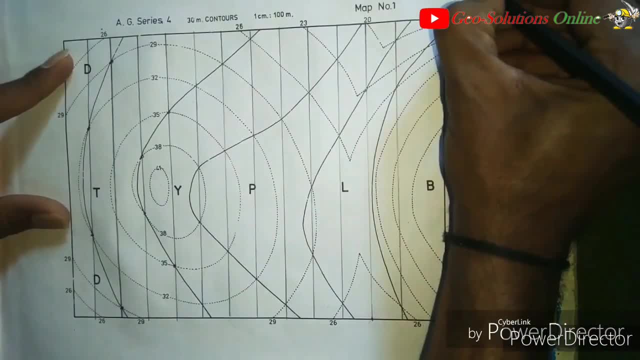 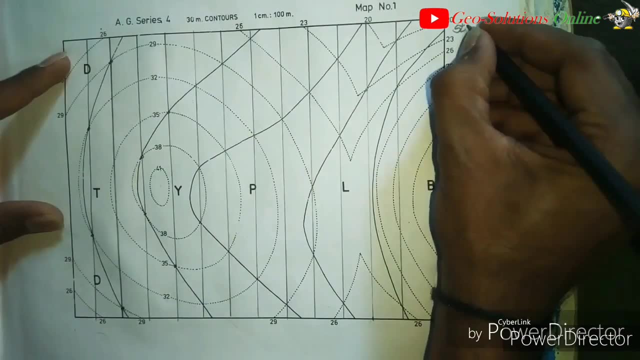 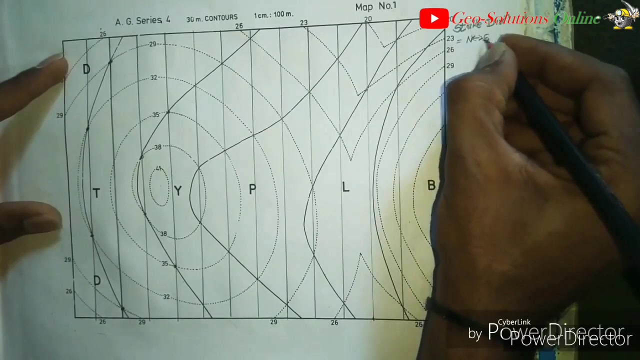 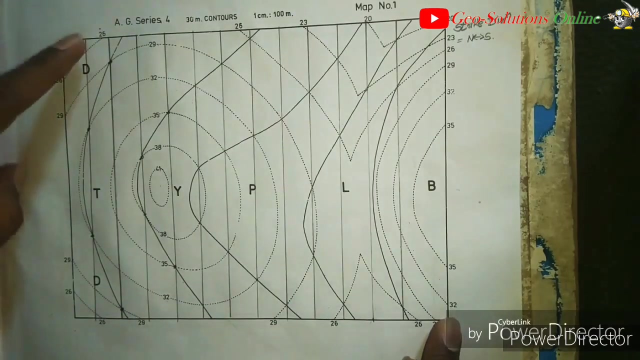 and the strike direction is: i will draw north arrow on this map. the strike strike direction is: i will write down here: is towards north, south. okay, so we have completed the strike lines on this map, number one. in this way, you have to draw all the strike lines. 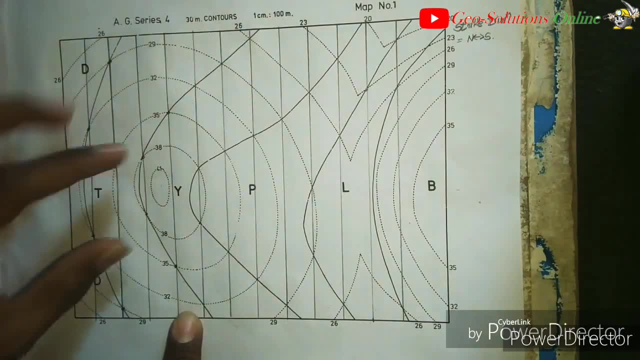 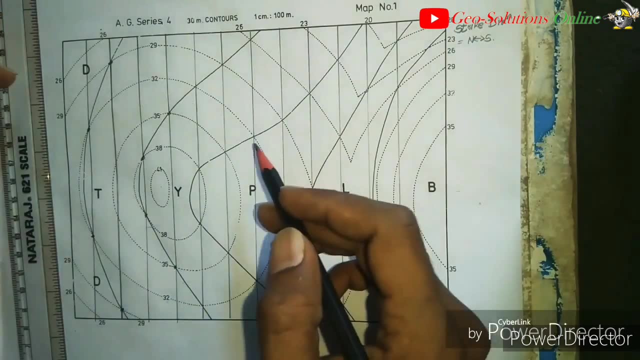 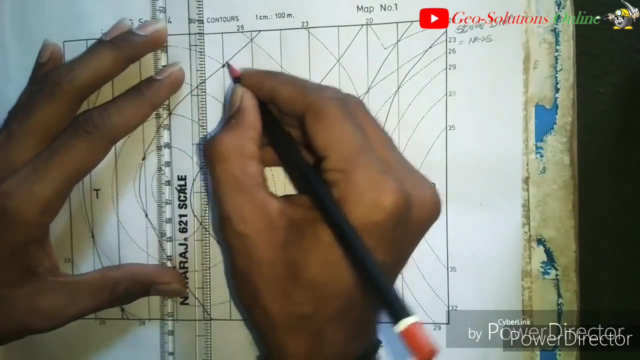 carefully by joining the intersection point in between same bedding plane and same control line. okay, but you can calculate the thickness of the bed with the help of the strike lines. but you have to consider a one strike line. okay, i will consider this strike line. so bed starting of the 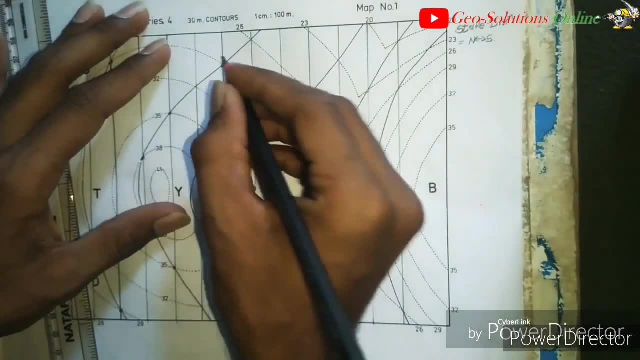 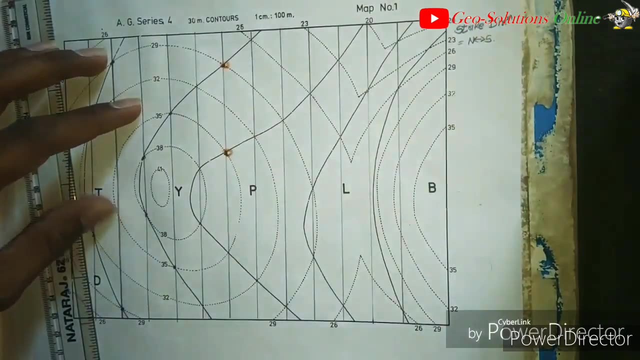 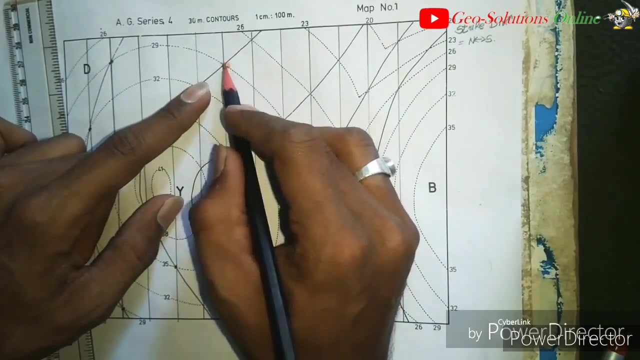 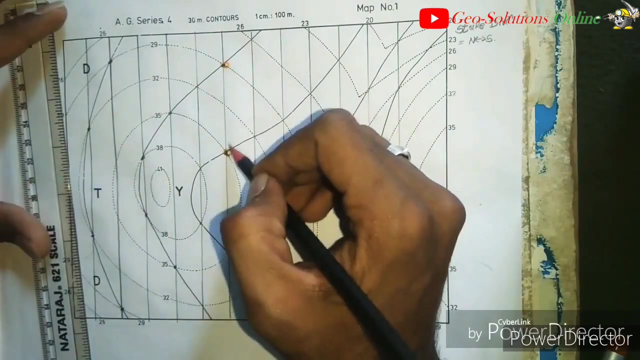 bed and ending of the bed, this intersection point of intersection. i will mark this point of intersection with this marker: okay, okay, these point of intersection where a, a junction point, junction line, contour line, a strike line, meets, that point of intersection is known as triple junction. okay, so consider two triple junctions on the beds and then measure. 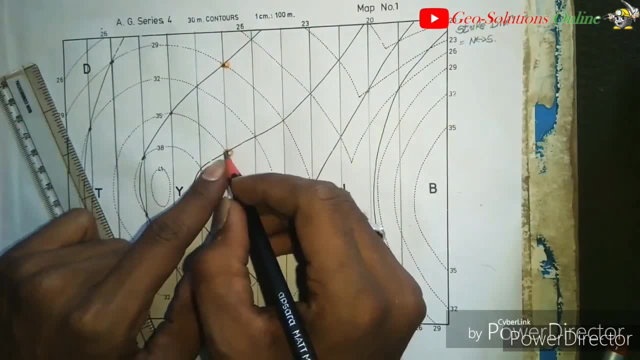 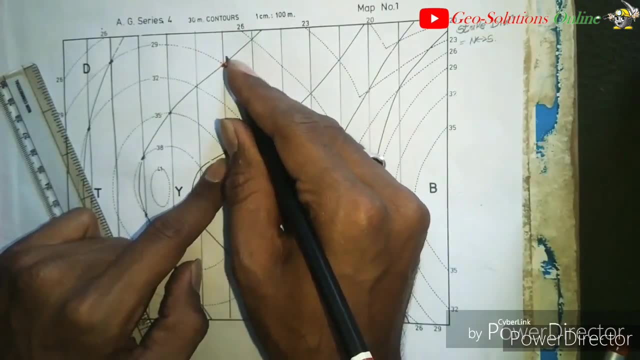 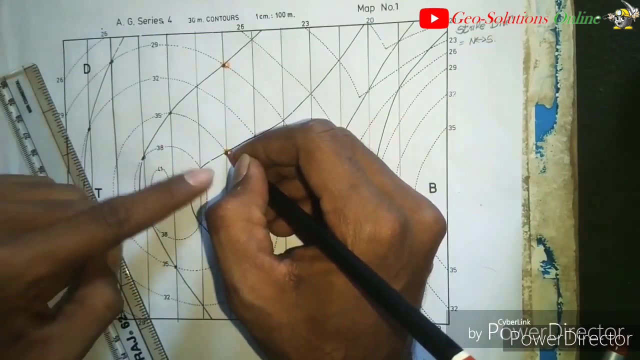 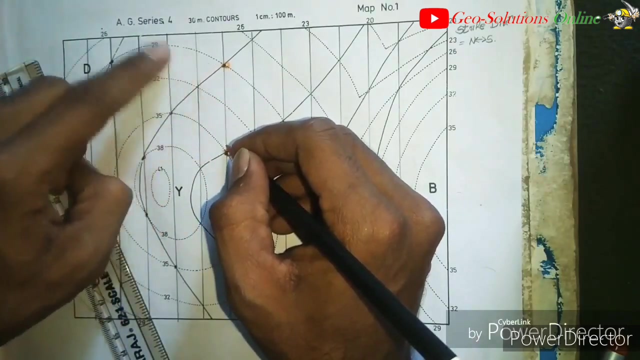 or calculate how many contours are going from that strike line: first, contour one, contour two and contour two, three. there are three contour lines going from this strike line in this bed y bed. then calculate: this is the contour line of 350 meter and this is the contour line of 2. 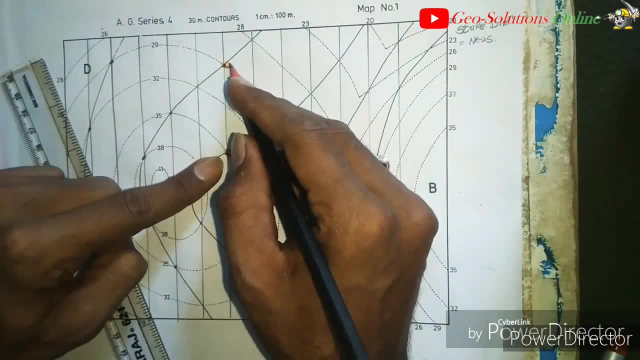 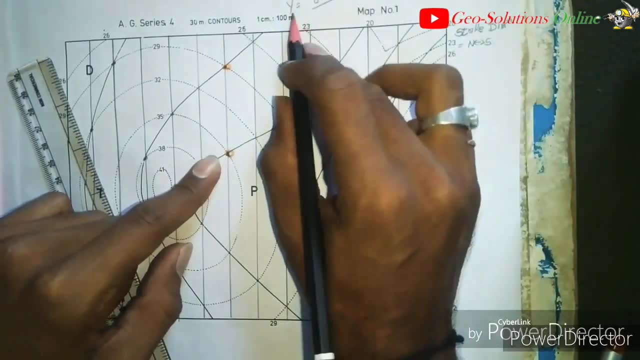 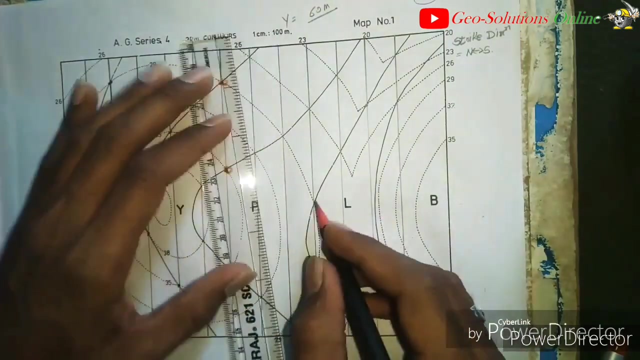 to 90 meter. so 350 minus 290 you will get the thickness of the bed, of the bed. so you can calculate of 60. that is, the bed y is having thickness of 60 meter. okay, bed y is having the thickness of 60 meter. then we will calculate the thickness of bed p. okay, i will consider this strike line and this. 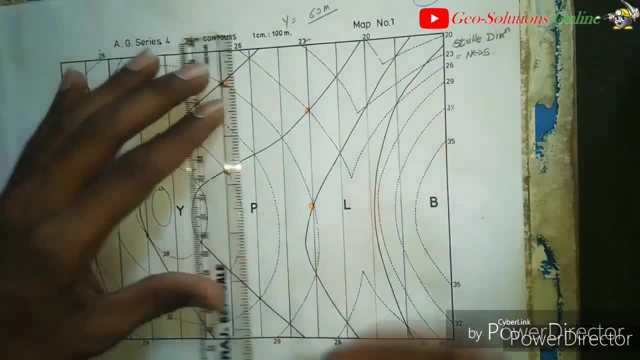 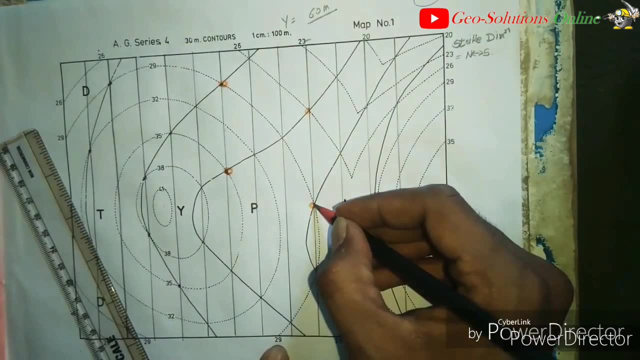 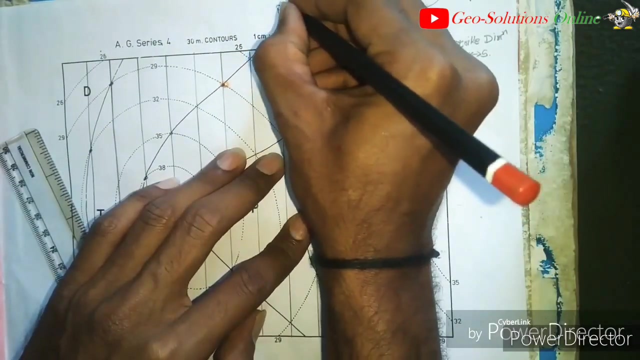 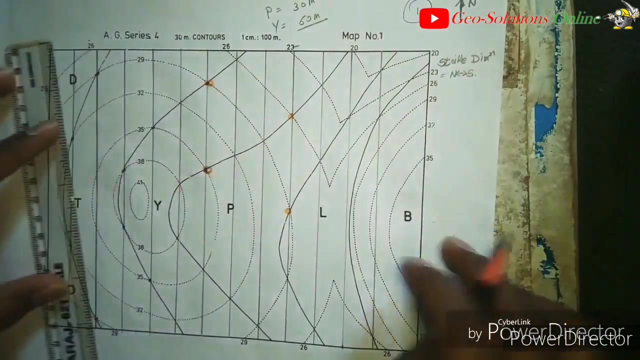 triple junction. okay, then, how many contour lines are going from this strike line? this contour is of 290 and this contour is of 260. so 290 minus 260, that means p bed is having this thickness of 30 meter. okay, now calculating the value of bed t, assuming that this bed is continuing. 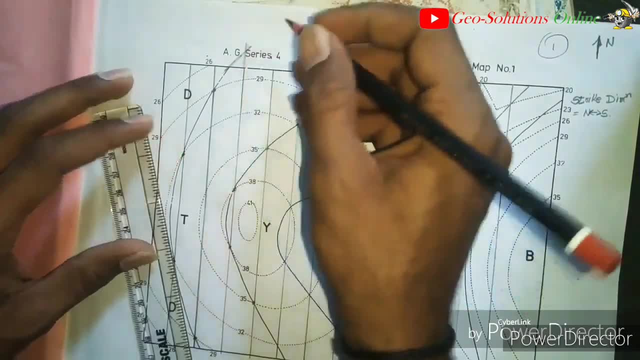 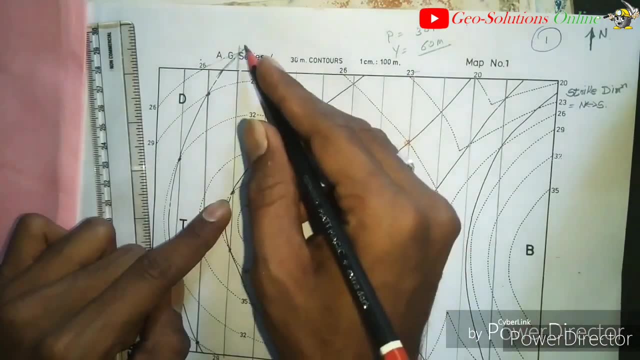 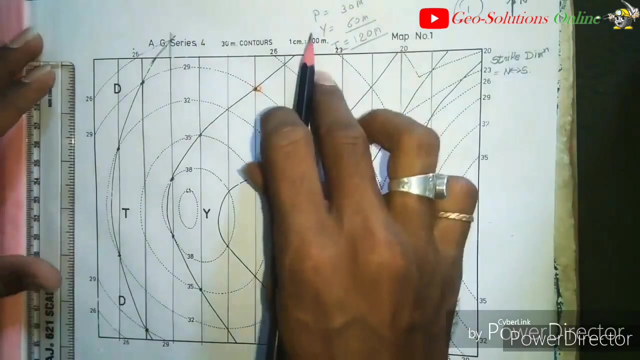 this and this is intersection, point of intersection, the maximum value of contour is having 380 and the angle is 260. so 380 minus 260 t bed value of 120 meter thickness. okay, in this way you can calculate the thickness of the bed with the help of this strike lines and 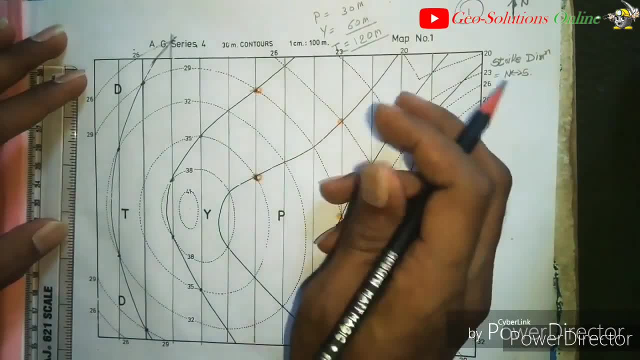 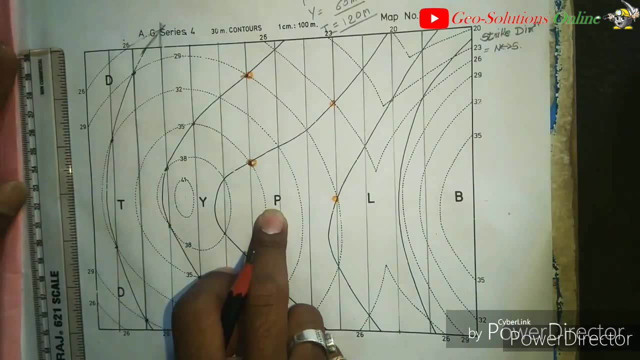 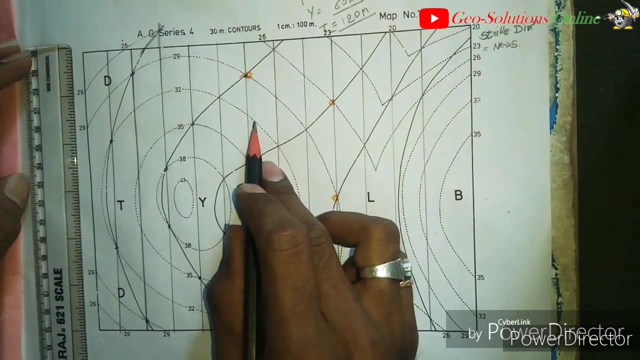 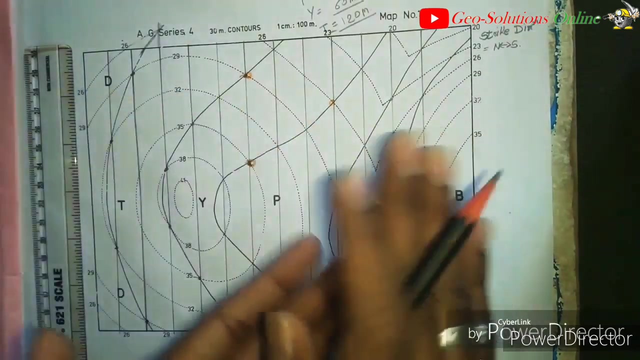 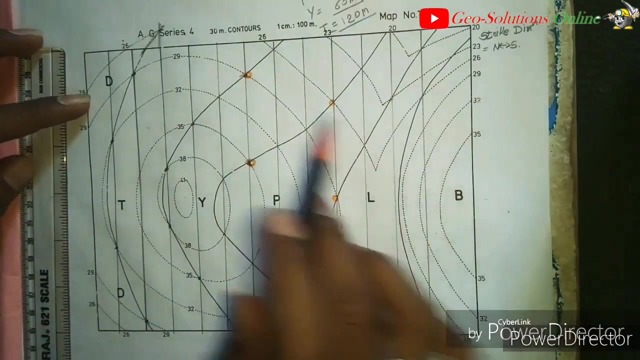 the bedding plane, or junctions. okay, so now how to calculate or how to identify the deep direction? okay, deep is nothing but the angle of inclination of this beds. okay, with respect to the horizontal plane. so that means in which direction these beds are dipping or inclining. okay, so these beds we are having, the beds of d, t, y, p, l, b. so if this, 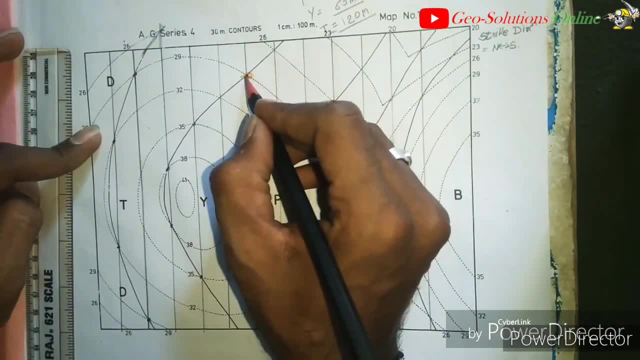 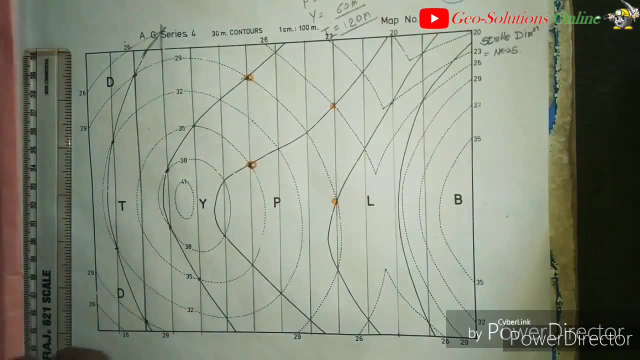 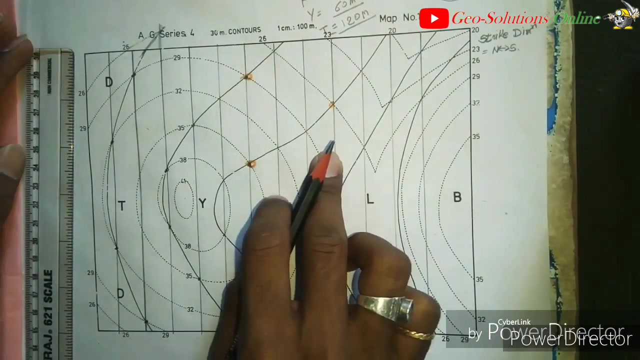 contour lines and this junction, junction points, are intersecting with each other, then it means the these beds are not horizontal, these beds are inclined in nature. so where this inclination is, in which direction the inclination is, we have to identify this. so the first rule for the deep 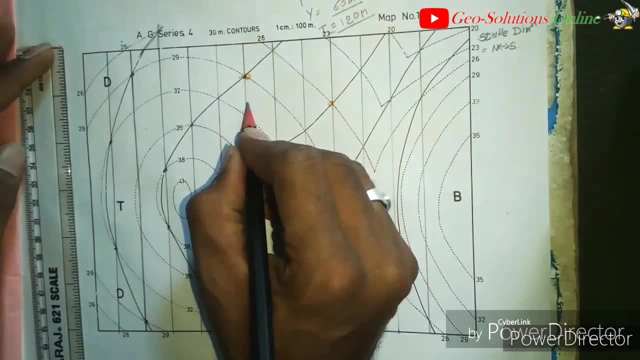 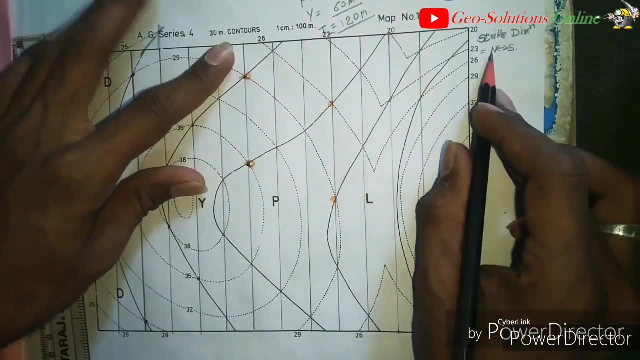 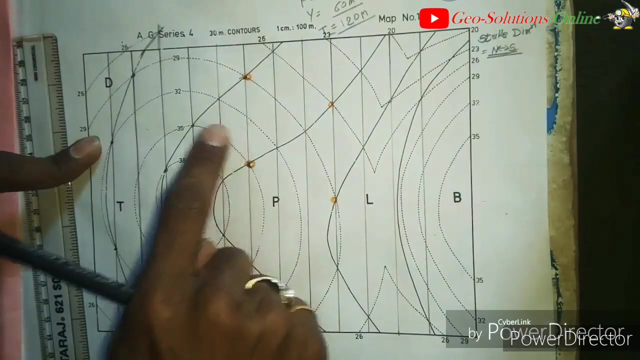 direction is deep. deep is always perpendicular to the strike line. okay, so consider this strike line. and deep is always perpendicular to the strike line. so we are having the strike line direction: north, south. so it means whether this beds are dipping towards west or whether these beds are dipping towards east. okay, this. 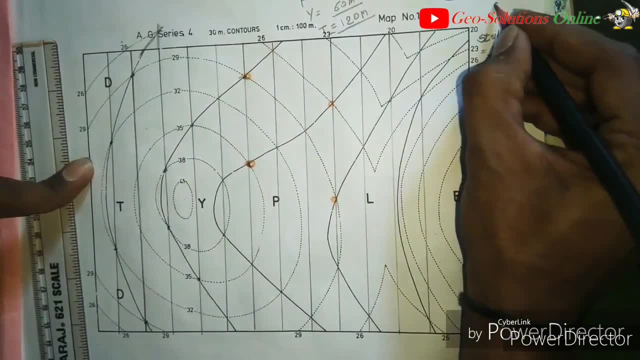 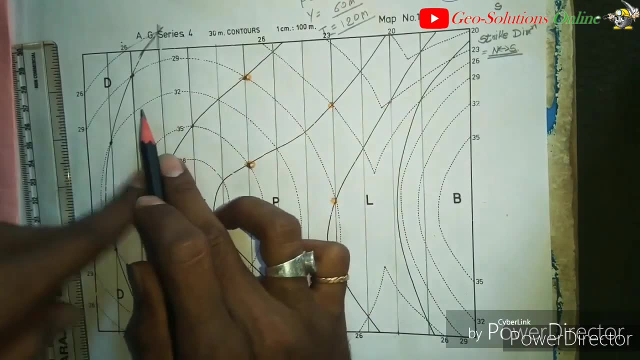 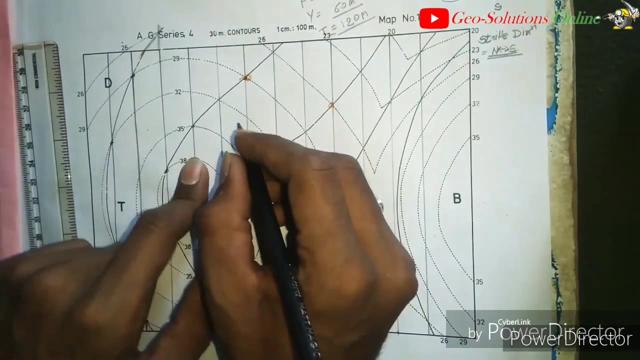 is east, this is west and this is south. so we have to identify that. so, whether these deep beds are dipping towards east or whether these beds are dipping towards west, because deep is always perpendicular to the strike line, okay, so, second rule of this: to identify the deep is considered three junction point. i will 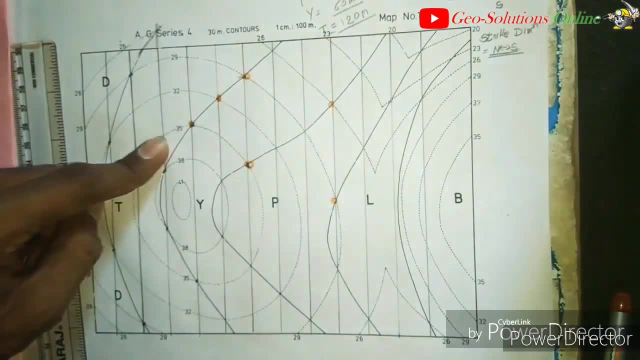 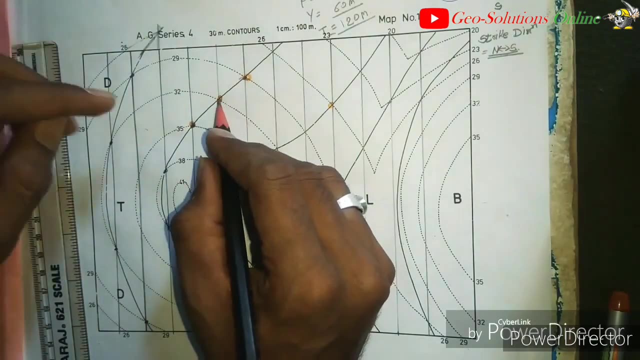 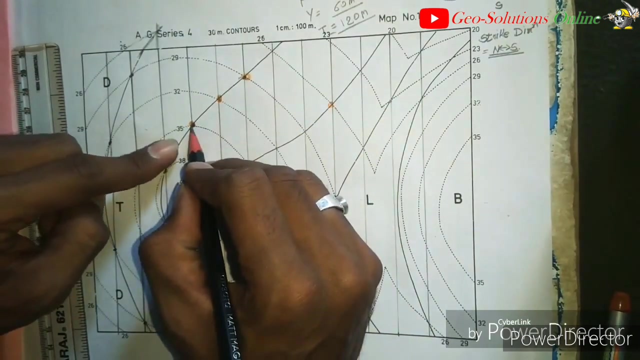 consider this three junction point, this three junction point on a junction line. okay, then i will consider this middle junction point and i will deep. second rule is deep always run from the higher contour to lower contour. okay values, okay. so this is the contour, this is contour is having value of 350 meter, this contour is having 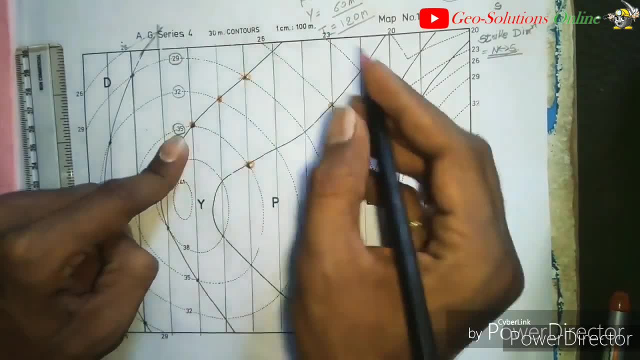 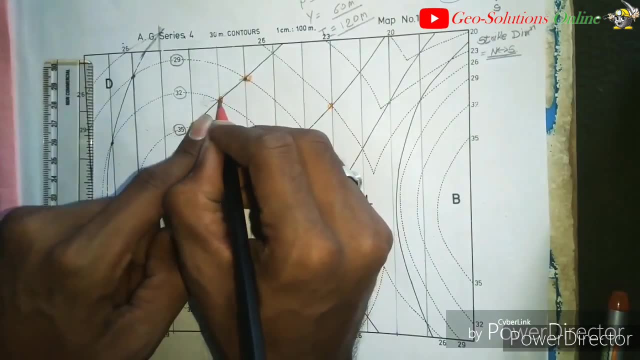 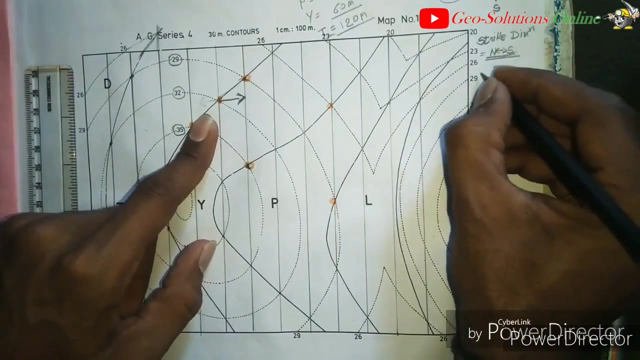 the value of 320 meter and this contour is the having the value of 290 meter. so i will consider this triple middle point, triple junction. okay, it is running 320 to 290 meter. that means the deep direction of these beds are towards the east, so i will write it down here: deep. 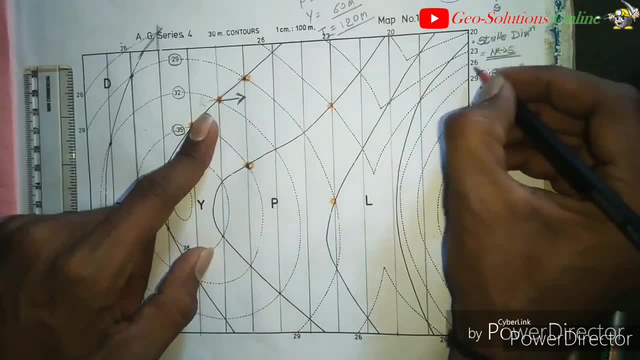 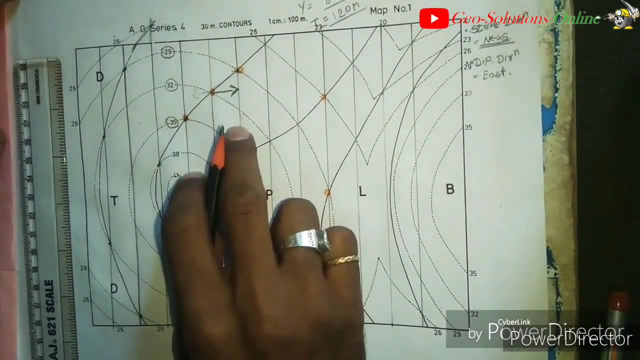 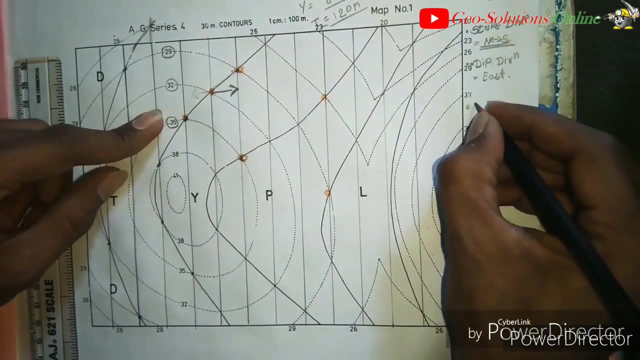 so we have find the strike direction and the deep direction. okay, so we have to find the. now we have to find the. we have already find the direction of the deep, and so now we have to find the amount of deep, and the formula of amount of deep is distance between 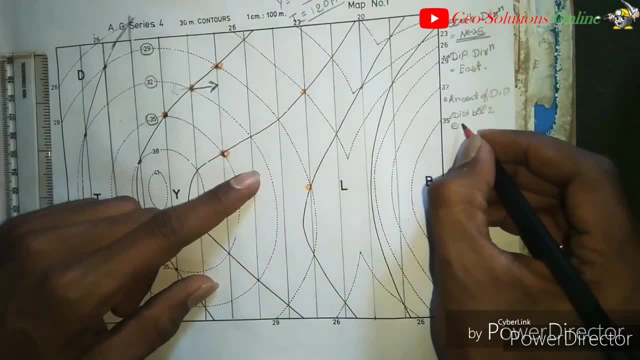 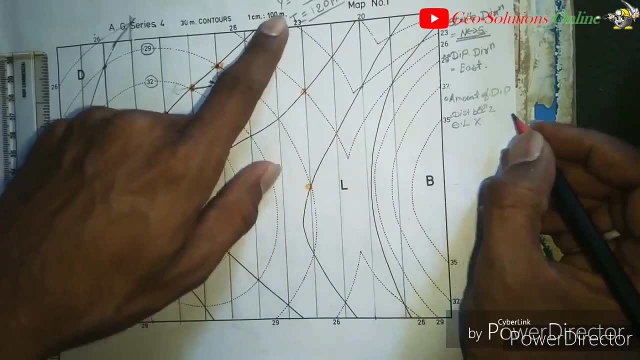 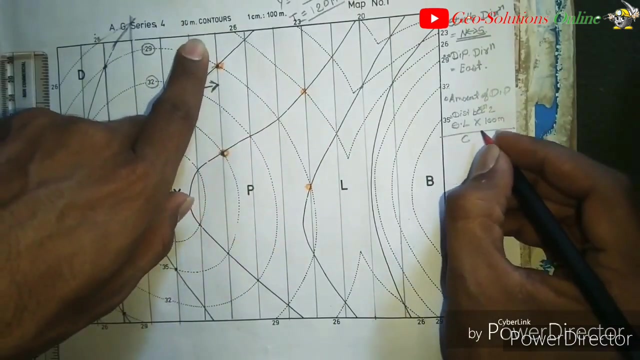 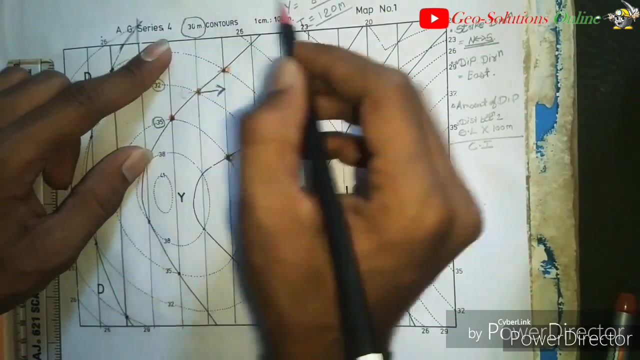 two successive strike lines- i will abbreviate that strike lines sl into scale of the map, that is 100 meter, okay, divided by contour interval ci, okay. so we are having the value of contour interval that is 30 meter, we are having the value of scale of map that is 100 meter and we 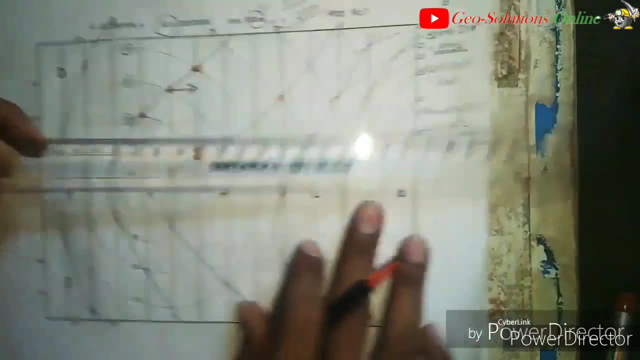 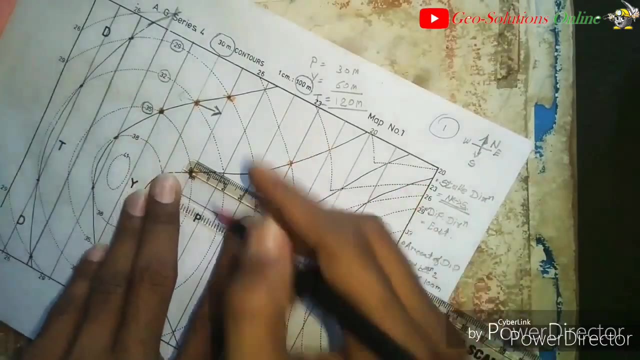 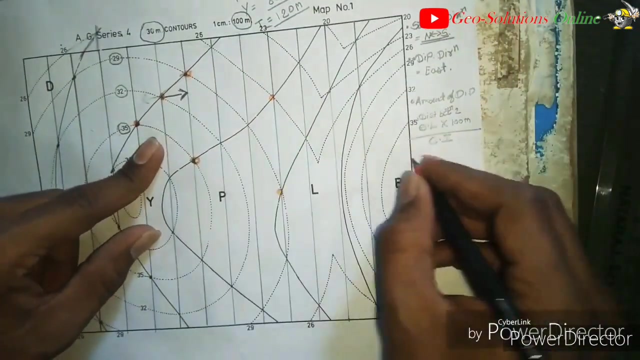 will measure the distance between two successive strike line, that is, i will consider these two strike lines. okay, here you can see: the distance between two successive strike lines is 1.5 meter. sorry, 1.5 centimeter. so i will write it down. write it down it here: 1.5 into 100. 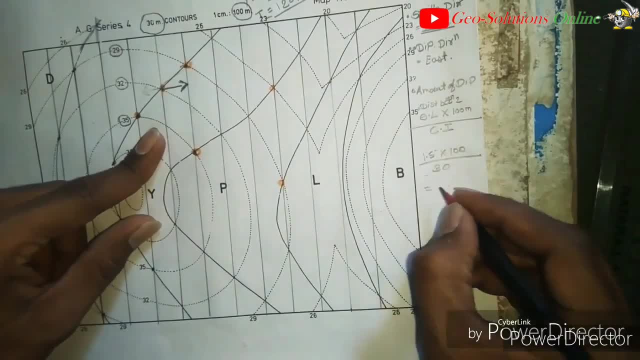 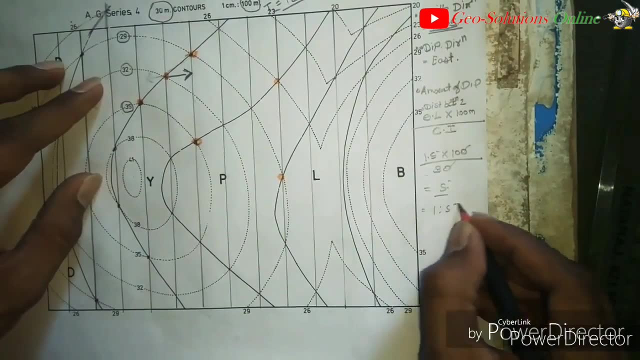 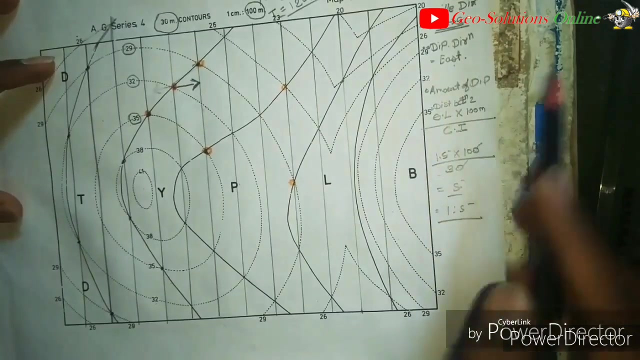 divided by 30, so we will have the value of five. considering this value in ratio, we will get one is to five. so deep amount is one is to five. okay, we have already find strike direction, deep direction and amount of deep, that is, angle of inclination with respect to the horizontal plane. 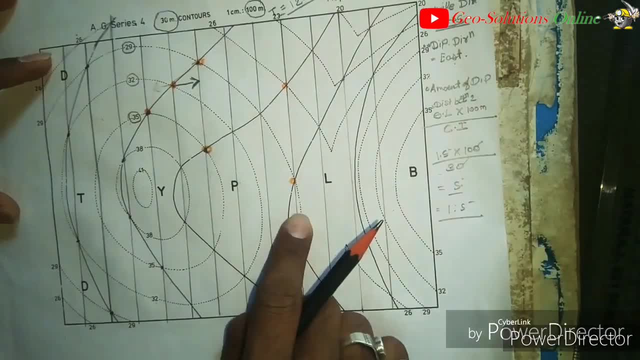 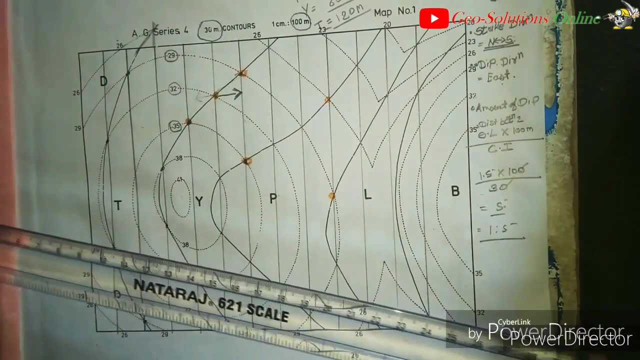 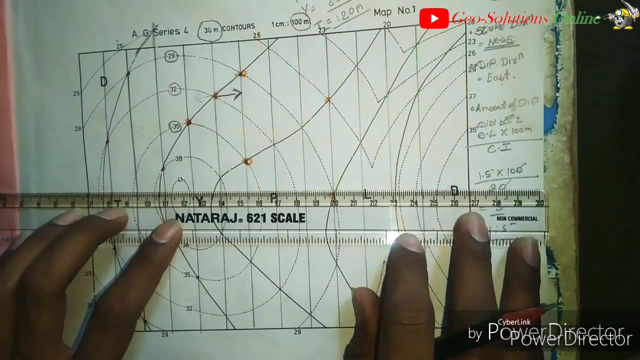 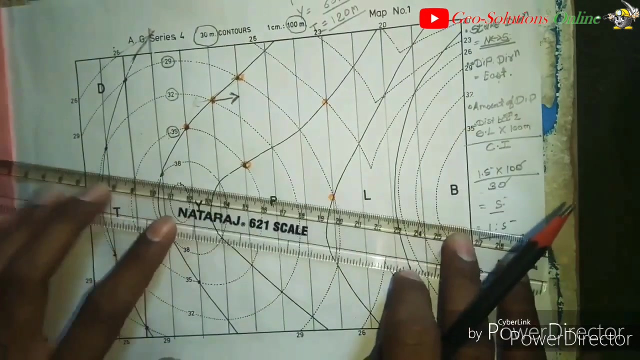 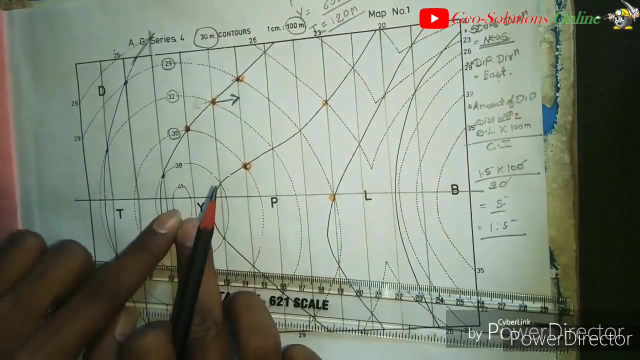 in in what angle these beds are inclined. okay, our next procedure of this map. you have to draw an axis, that is axis XY, to plot the section. so I will draw a axis XY in such a way that it will cover all the geographical features on this map. so I will draw the axis from here. it will cover a isolated hill, a saddle and 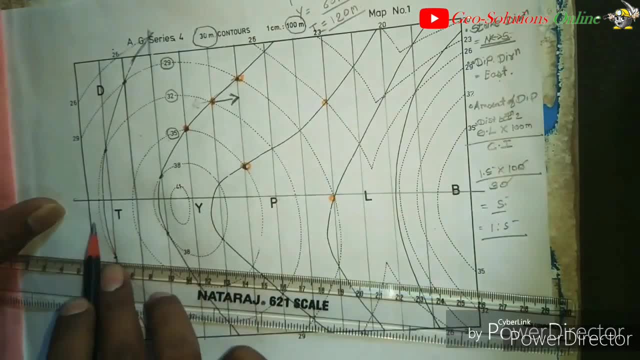 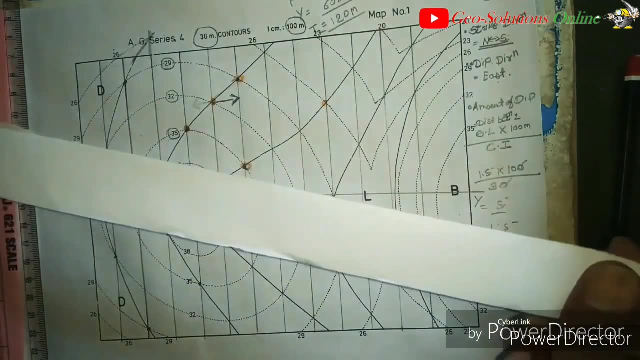 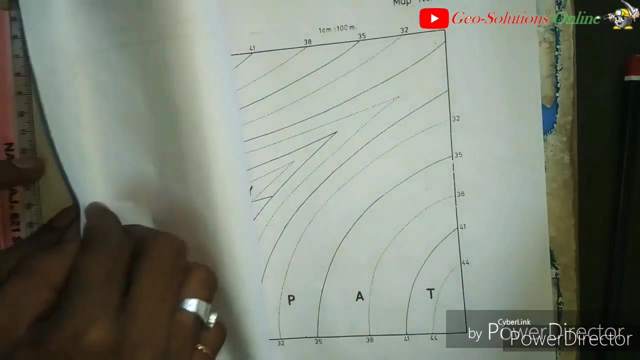 another isolated hill and all the beds okay: bed D, bed T, bed Y, bed P, bed L and bed B. you have to make this type of a strip of a paper, get the center point of the paper and get the center point of this. two axis points okay, like this: 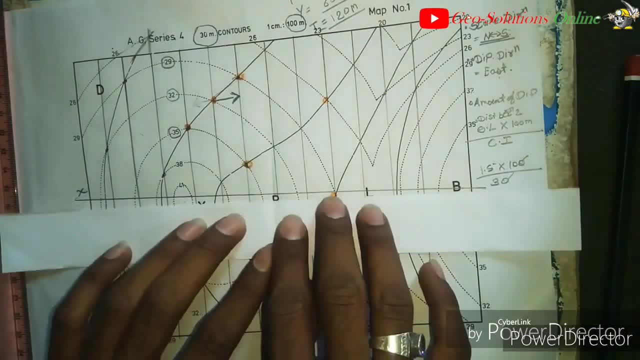 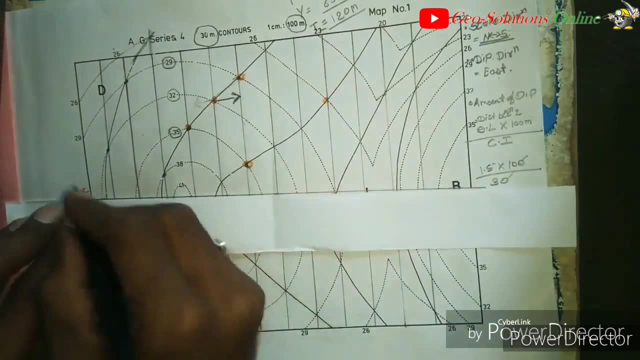 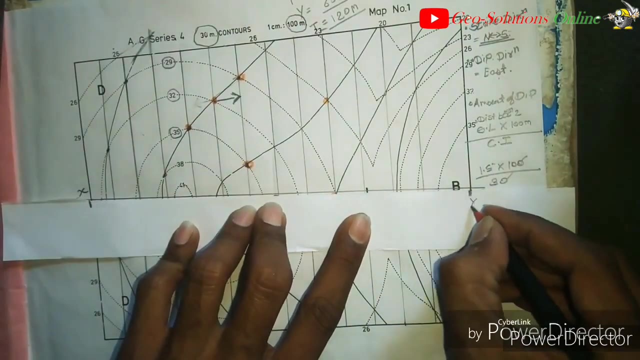 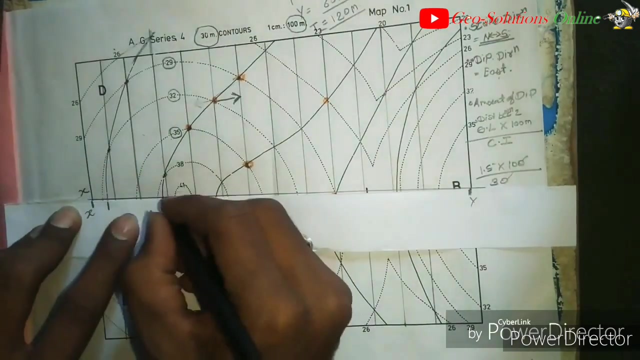 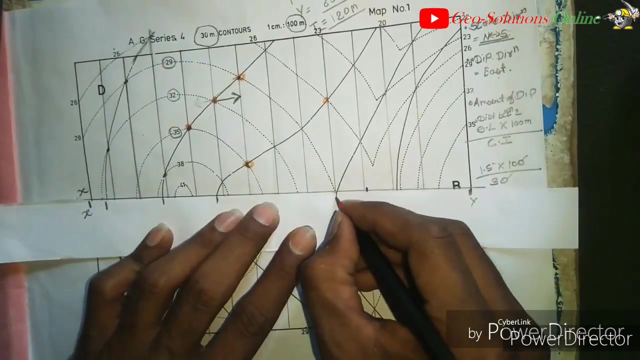 center point of the map and center point of this, your strip. keep this streak paper like this in this manner: on the XY axis, mark the X point and mark the Y point carefully: Y and X. then you have to mark all the junction point. first I will plot this junction point on the strip paper label. 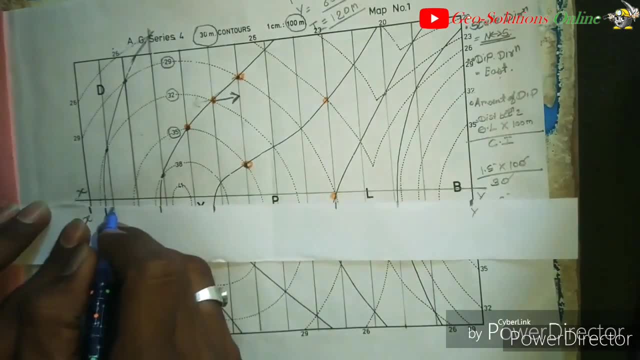 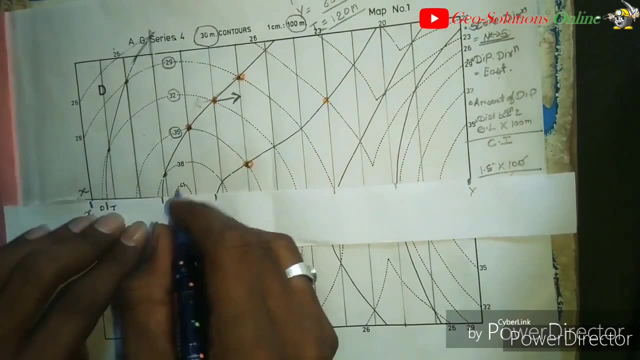 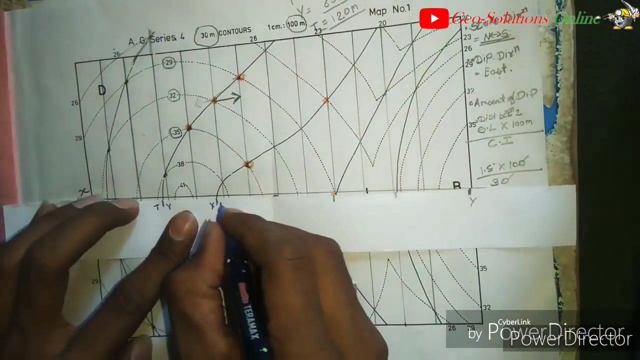 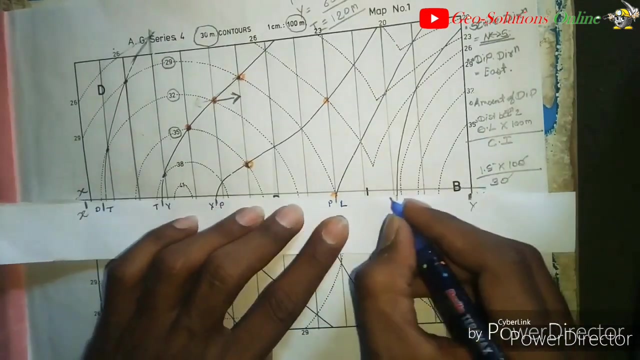 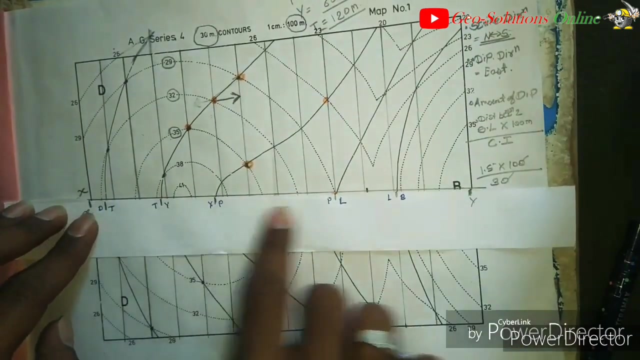 it carefully with the help of a pen to avoid the confusion. okay, theды junction, this is the 在. this is why 하나, and this is we tension, and this is, and we change. okay, so I have already plotted XY point and all the tension points. now we have